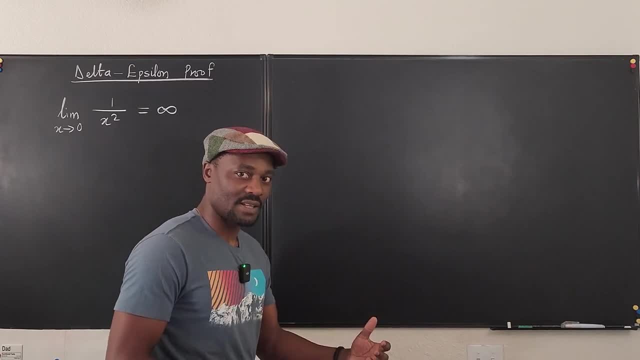 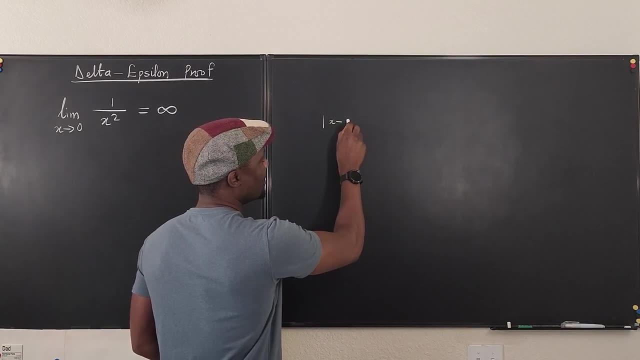 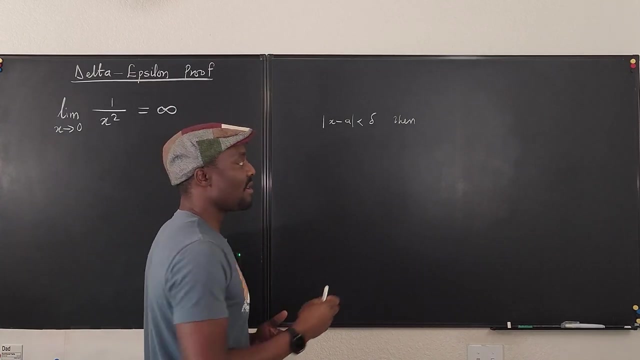 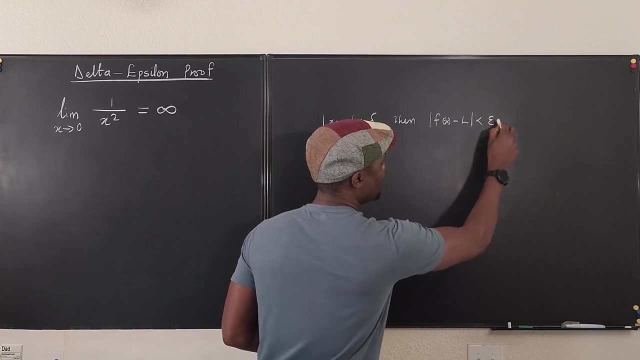 epsilon greater than zero and for every delta greater than zero. if the absolute value of x minus a is less than delta, then we have the absolute value of f of x minus l is less than epsilon. This is typically what we write for epsilon and delta. 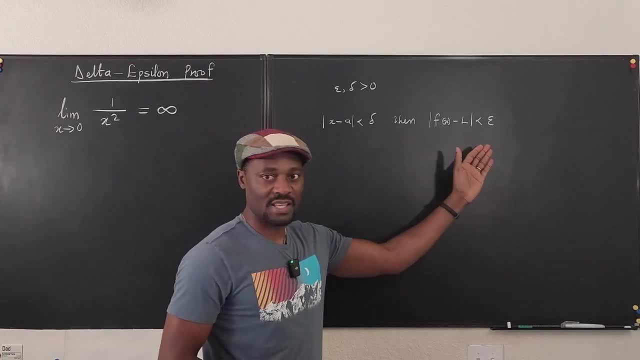 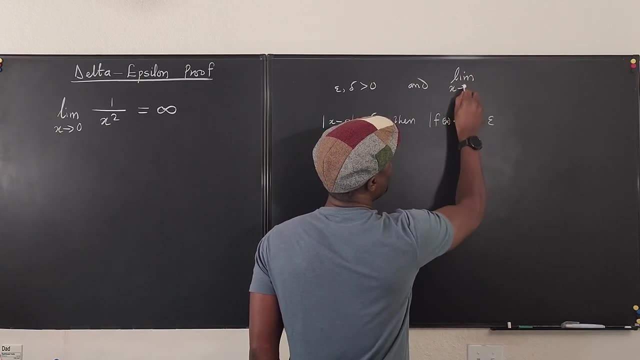 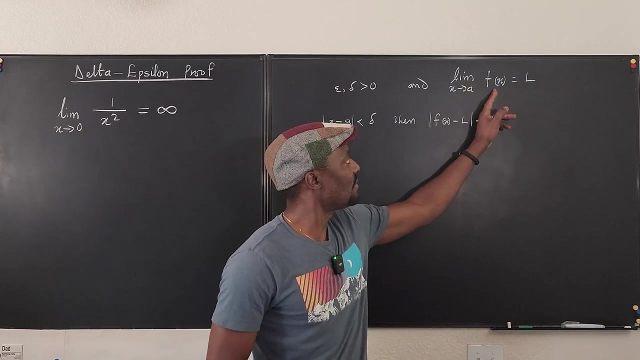 greater than zero. Okay, we say this is the case if we have this, claim that, and we say that the limit, as x approaches a, of f, of x is equal to l. This is what we usually state: that if the limit of this function is l, then we can say that if x minus a is less. 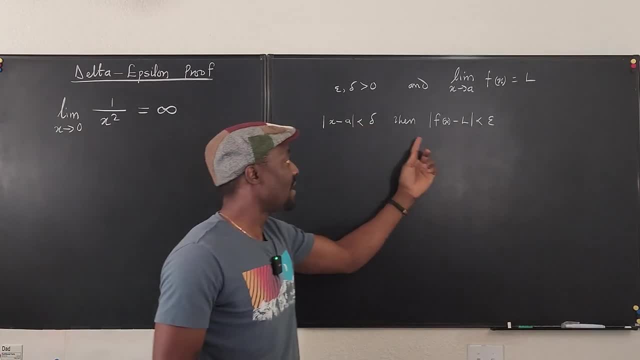 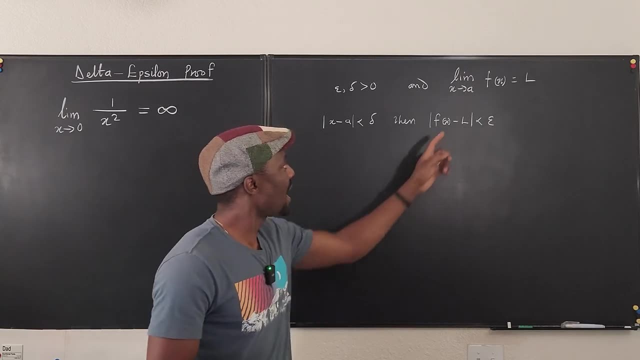 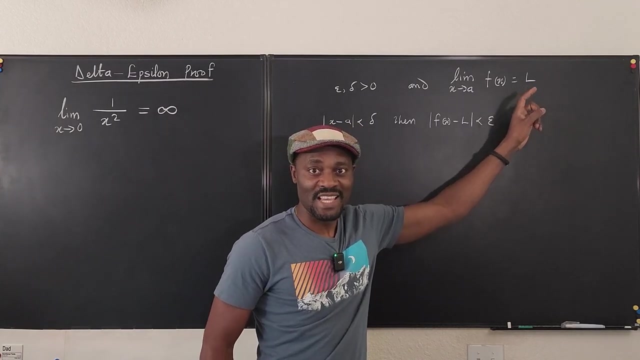 absolute value of x minus a is less than delta, then f of x minus l is less than epsilon. The problem with this, using it here, is that we do not have a finite limit. Okay, and because we do not have a finite limit, it is impossible for you to say: okay, I know what l is, because 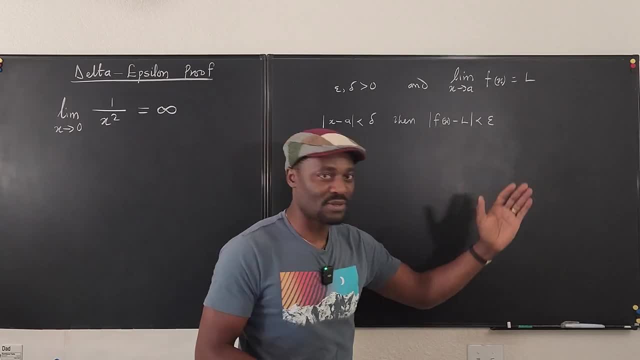 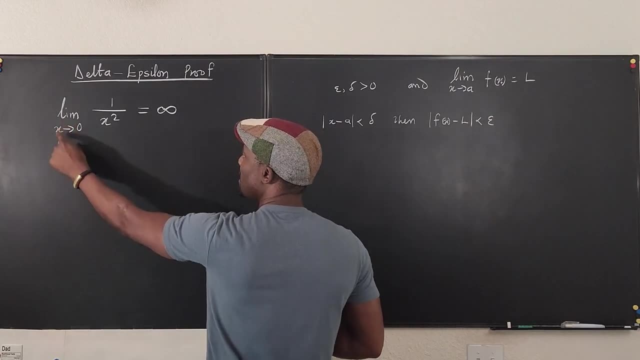 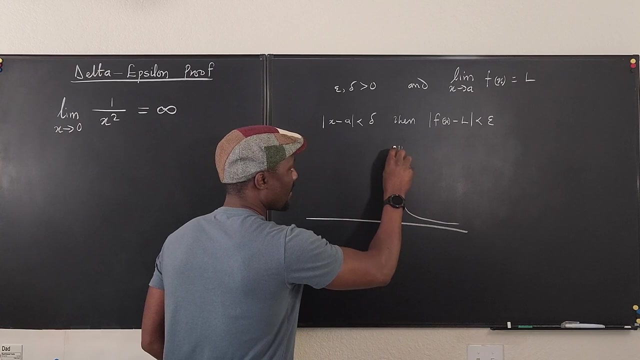 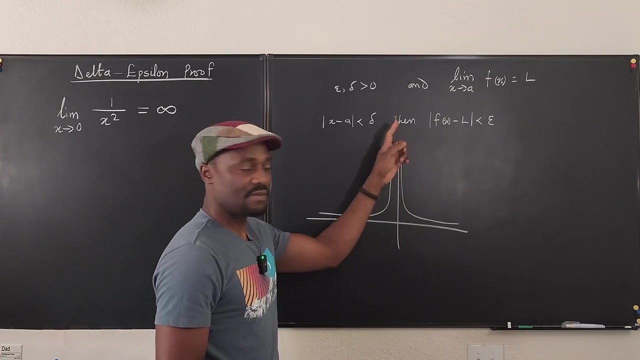 infinity is not finite, So this definition will not work. This is the definition you should imagine. Look at the function that we have. We have the limit of 1 over x squared. This is what we have And you notice that the limit from the right is positive infinity. The limit from the 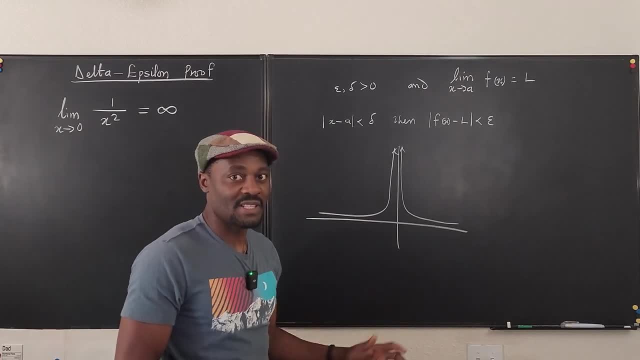 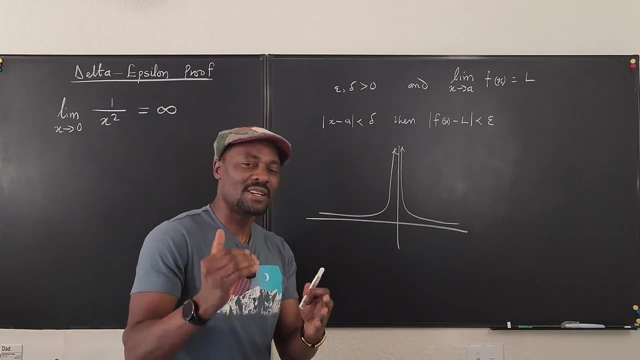 left is positive infinity. So we say that the limit of this is positive infinity, which means if you can imagine a number, no matter how big the number is. so let's say 247 billion. Okay, if you get close enough to zero, you can imagine that the limit of 1 over x squared is: 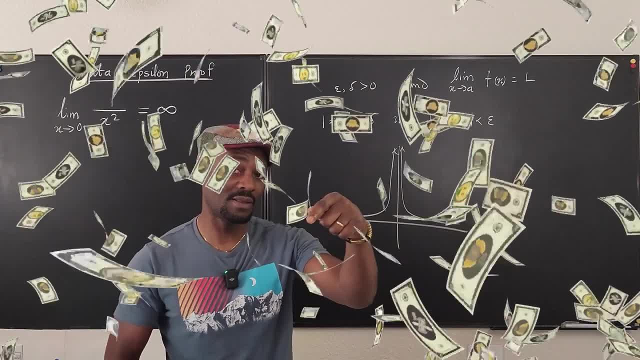 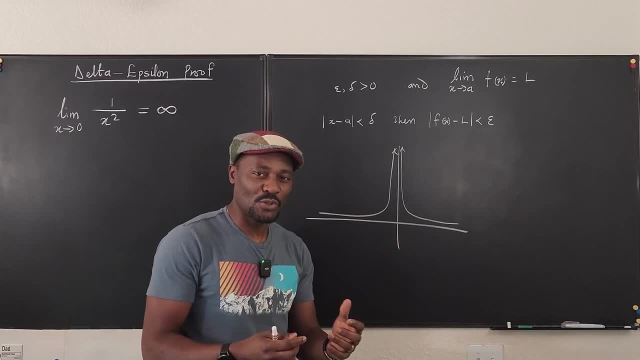 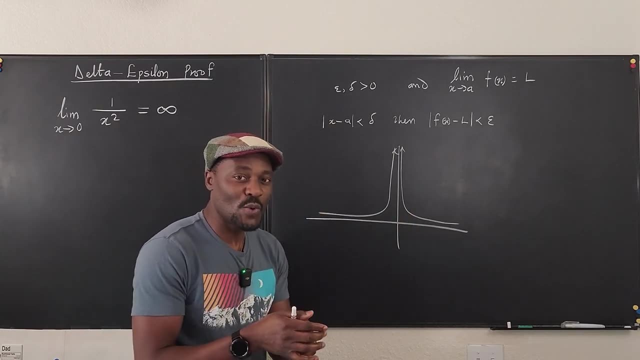 zero. The limit of this function will still be greater than that number- 247 billion- because the limit is infinity. We just want to be able to show that if you stay close enough to zero, your limit will be infinity. So we're trying to be as close as possible. So our delta is going to be very small. 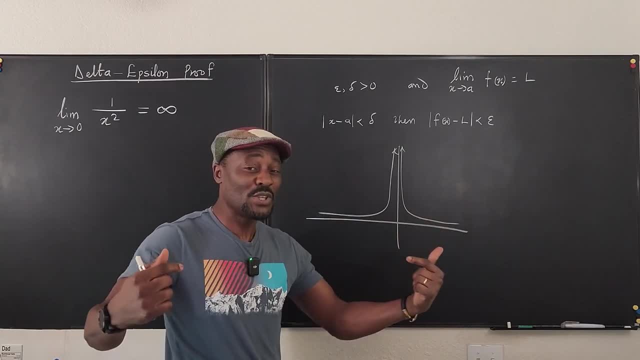 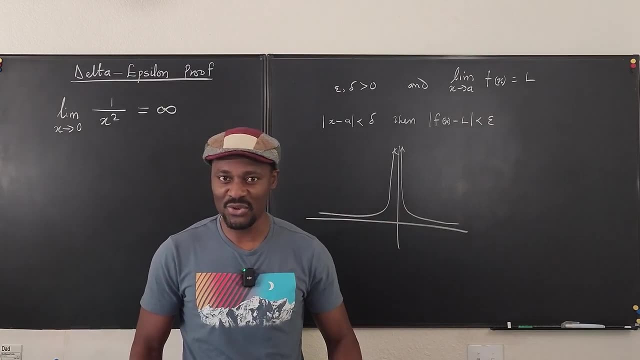 Whatever number you can imagine can be as big as anything. We just need to prove that if delta is small enough, the limit of this function will still be greater than that number: 247 billion. This function will be bigger than any number you can imagine. 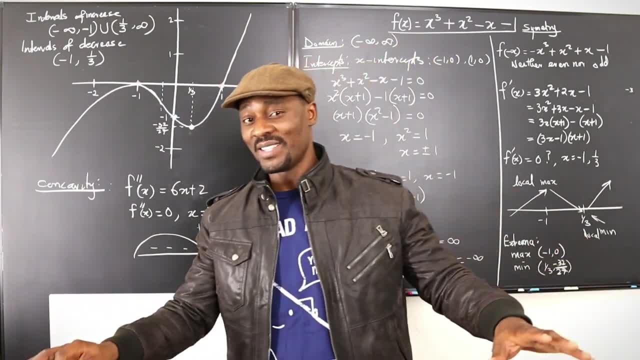 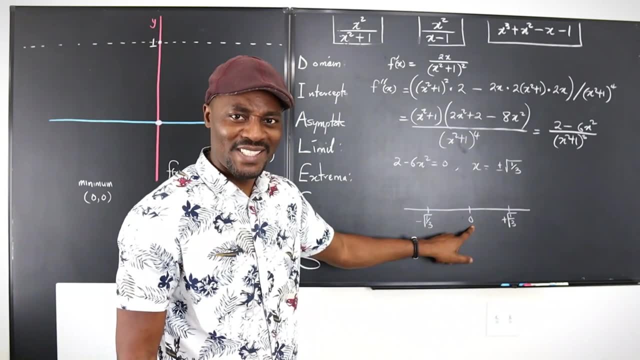 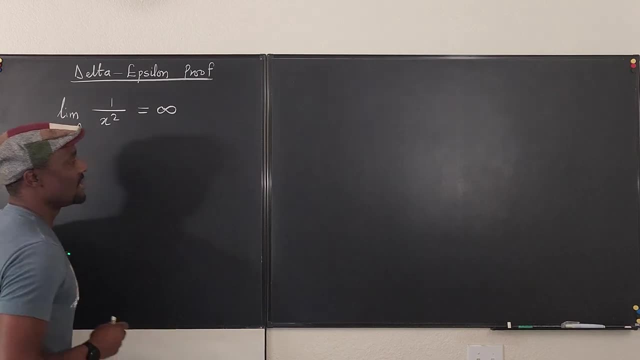 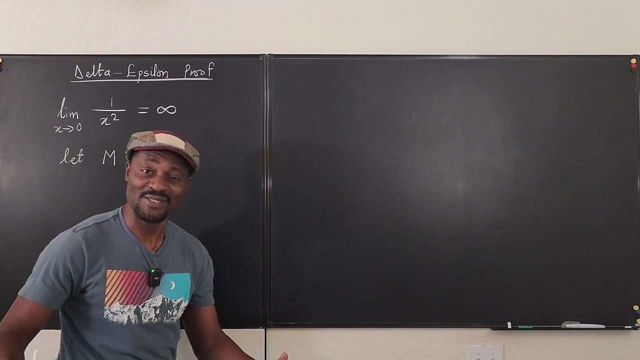 Let's do it. So this is what we're going to do. We're going to say: hey, let's imagine a number. We say let a big number. Let's say let m. Let m be a number we know that is greater than zero, m. is that number 247 billion, right? I don't. 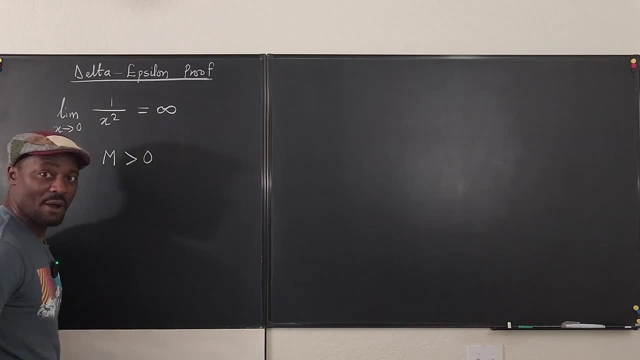 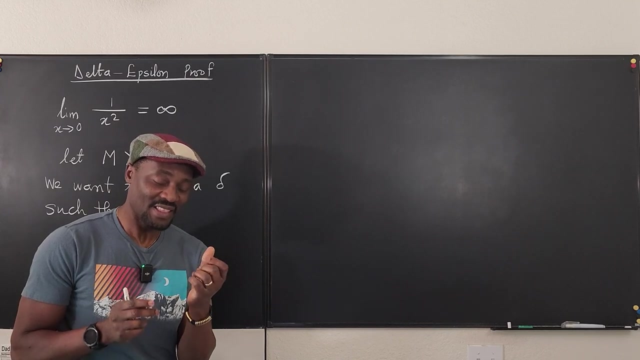 know why that number keeps coming to my head, but let m be that number Now. we know. What we want to show is that there exists a delta. We want to show, we want to find a delta, Pl왔j that if θ is small enough, okay, That is the gap. 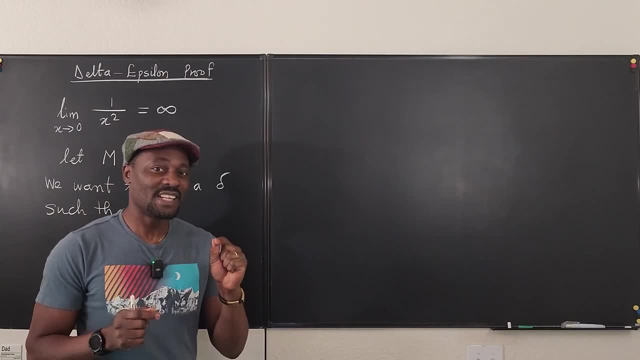 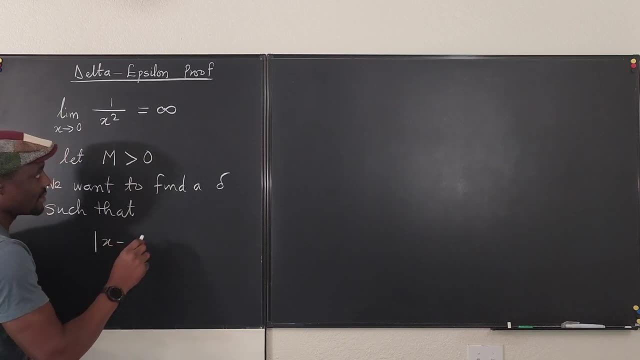 between x and zero is less than delta. this way, if the absolute value of x minus zero Gi delta is less than delta, That is, if delta is small enough, this gap between z and the xtan of the empty, 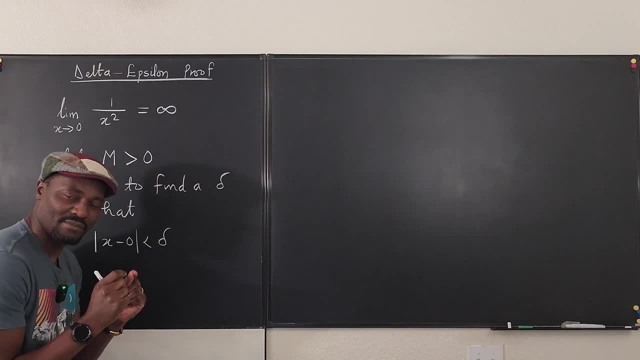 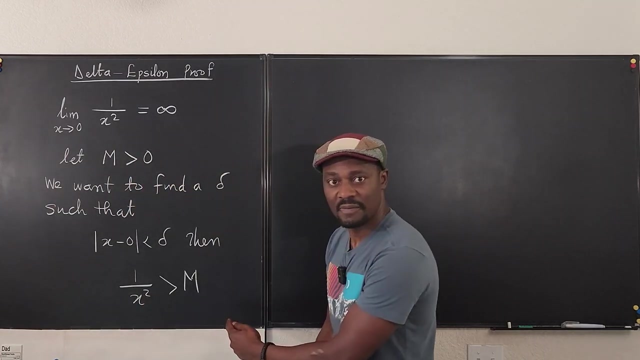 gap is small enough. we're looking for that small gap. If we can get this delta, then this limit, 1 over x squared, will always be greater than this number we're talking about. I've already explained that, but this is the sentence: That if delta is small enough, 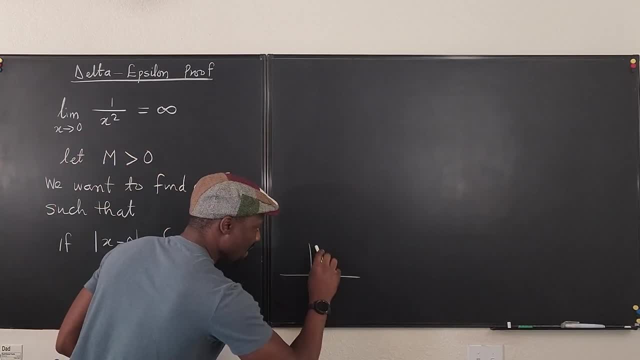 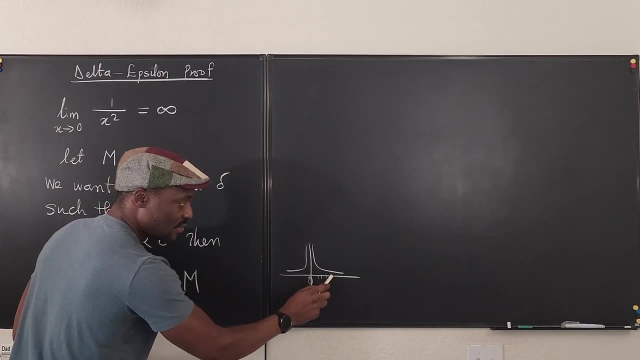 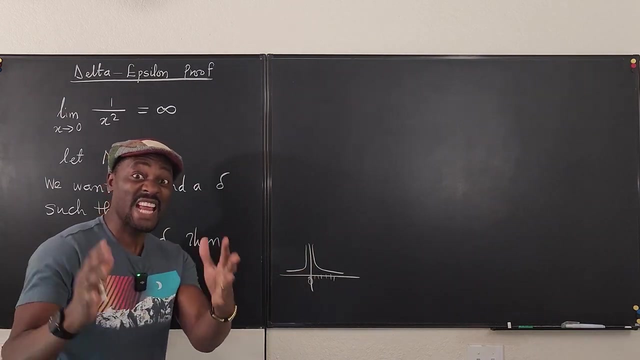 that is the distance of x. Look, So this is 0.. This is where we're calculating the limit. If the values of x you're using are close enough to 0, then the limit you're going to get for this function will be greater than any known number. 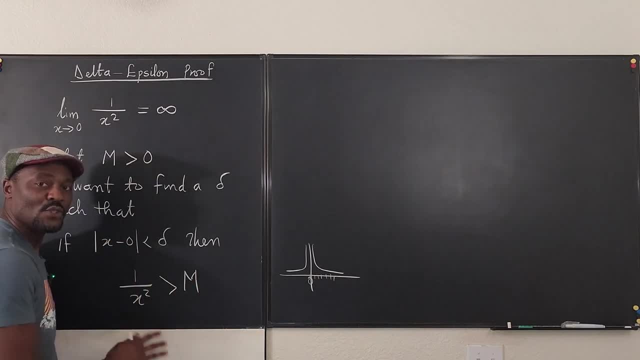 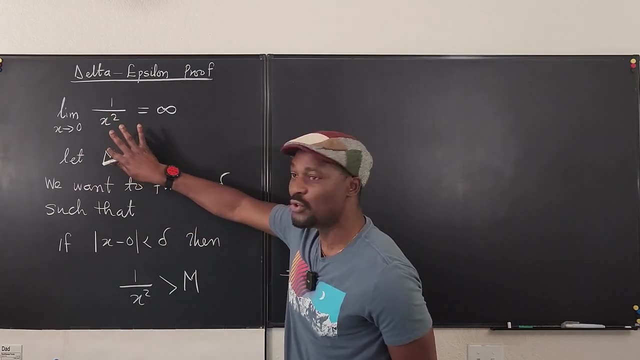 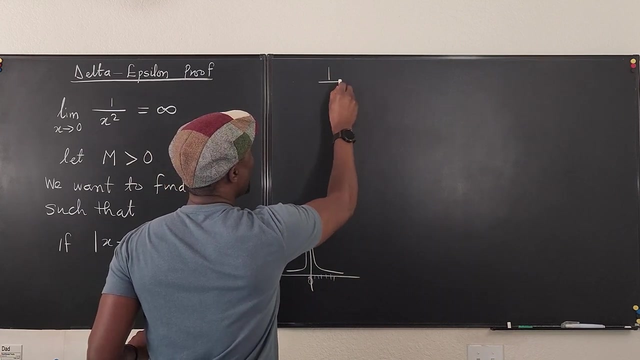 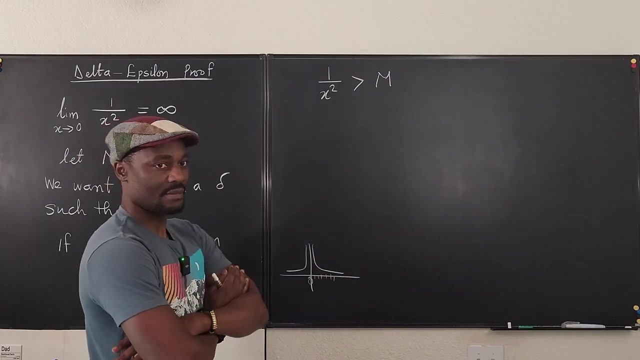 That you can imagine. That's the concept here. So how do we show that? Well, this is what you do, The same concept. You manipulate what you have to get what you want. So what we're going to say is: let's go here. If 1 over x squared is greater than m, what do you see? 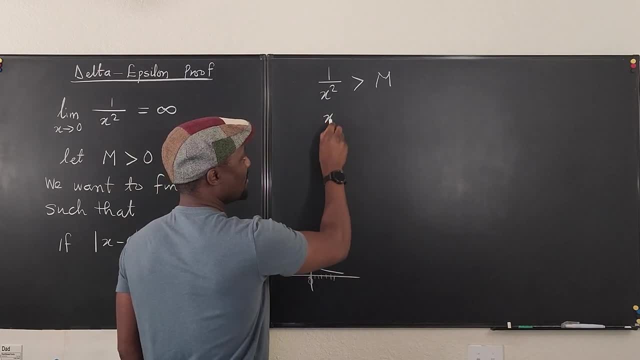 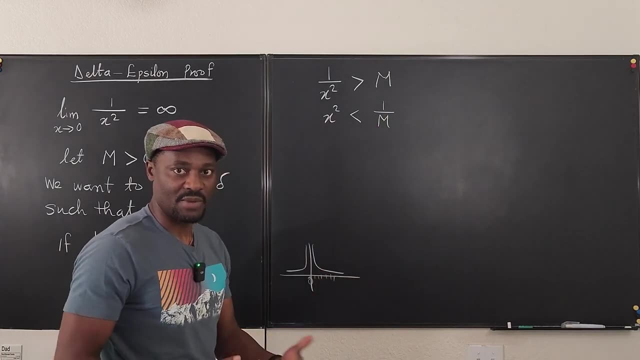 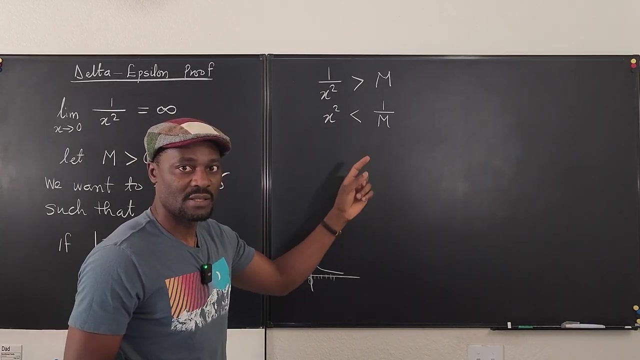 If we flip this, we know that x squared will be less than 1 over m. That's a basic principle of inequalities, right? But we don't want x squared, We want to take the square root of both sides. If you take the square root of x squared, what do you get? It's the absolute value of x. 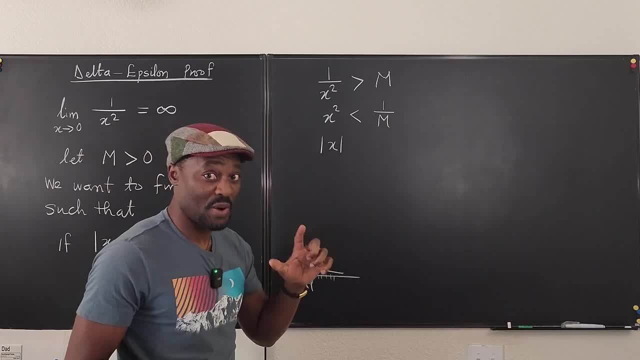 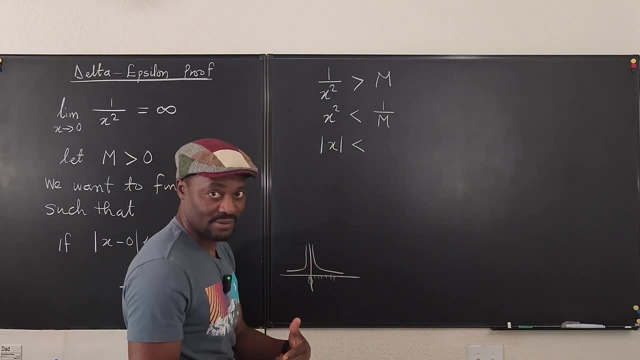 I've often said this in my videos, that the square root of x squared is the absolute value of x. That's why on this table we have x squared. So we're going to take the square root of x squared And on this side we usually get plus or minus. Okay, So this? 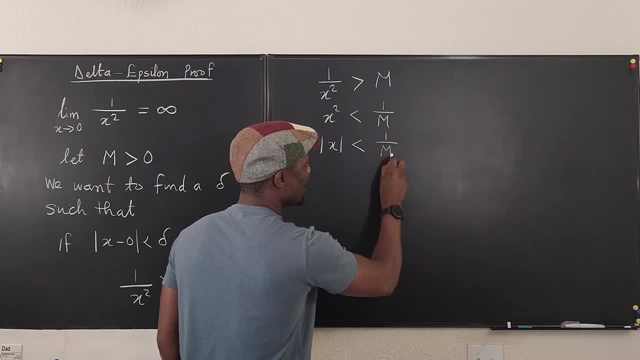 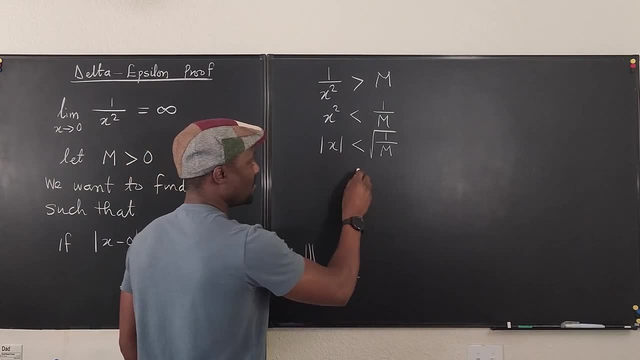 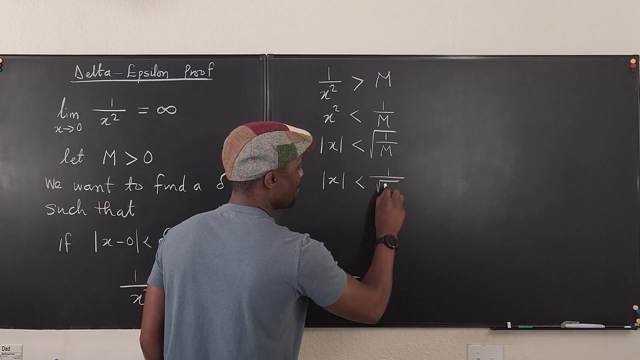 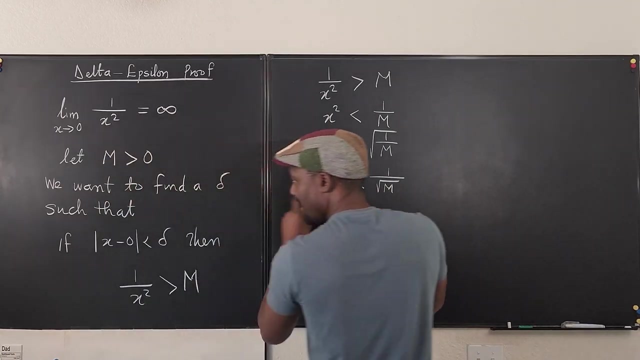 is 1 over m square root, So well, the square root of 1.. So we can just say that the absolute value of x is less than 1 over the square root of m, Or you can leave it this way. But look at this This: 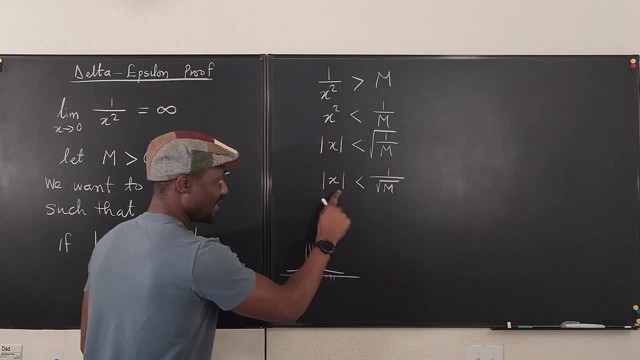 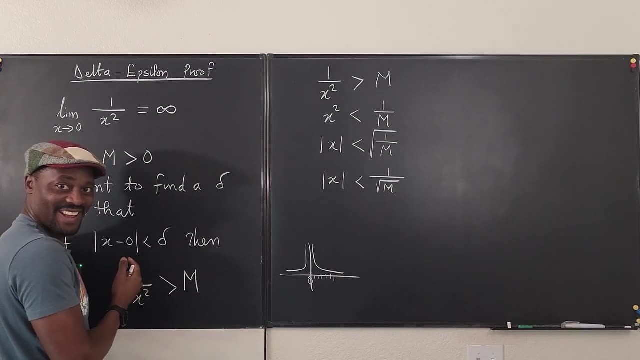 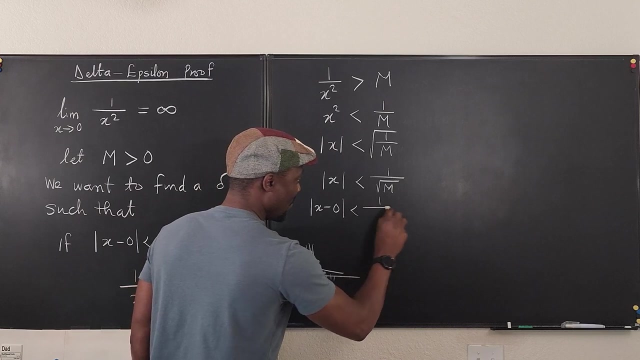 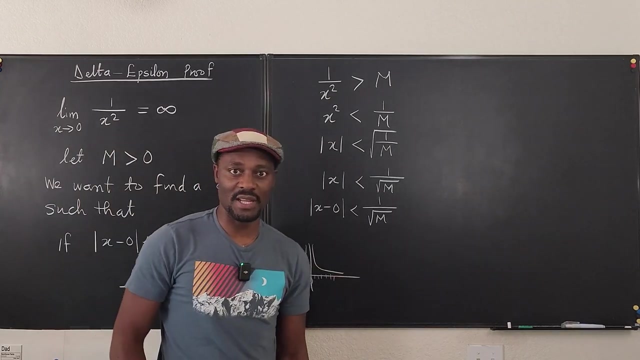 is 1 over m square root of m. That's this. I can actually rewrite this expression to be x minus 0.. You can see that. So actually I can write this as: x minus 0 is less than 1 over the square root of m. So now, clearly, I can claim that this is the delta I've been 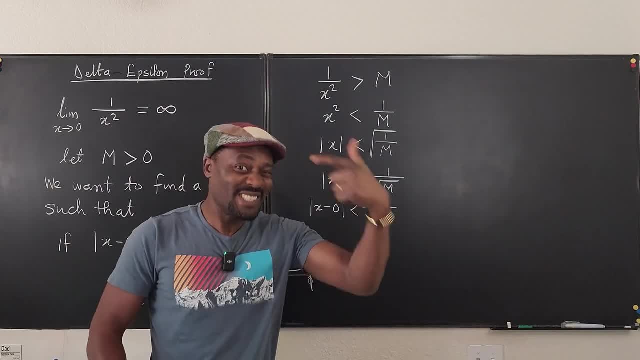 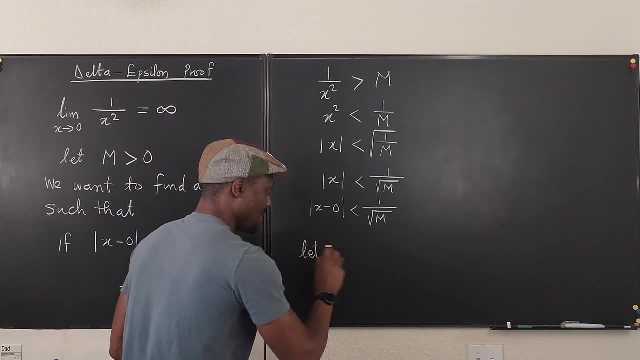 looking for 1 over the square root of m. There exists a delta, And once you've found the delta, you're done with your proof. I'm going to now say: let delta be equal to 1 over the square root of m. That's it. This is all I need to show. 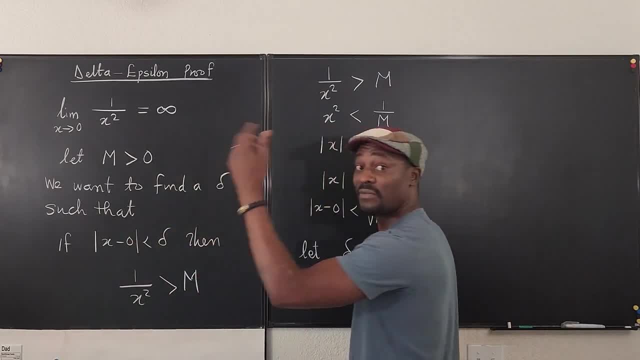 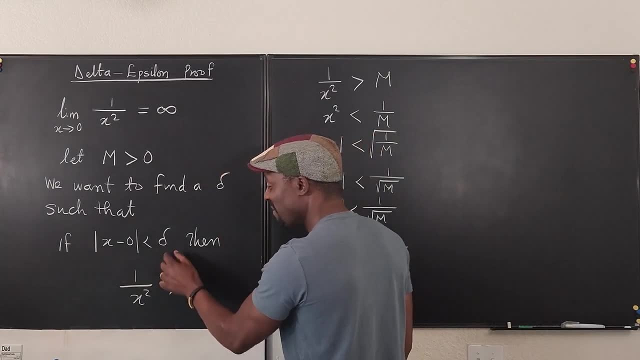 Okay, Once you have this, go back to the claim from the beginning. What was the claim? This was the claim That if we can find a day, if we can find a delta, we want to show that we want to find a delta. We want to find a delta. We want to find a delta, We want to.